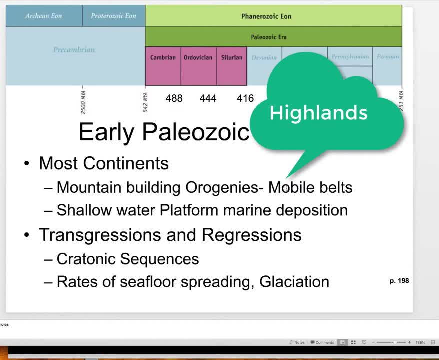 So these mobile belts are highlands, where there are compressional activities, really just along the margins of the continents, as new terrains, new land masses are being accreted or attached to North America And we call those orogenies. Remember oro means mountain and so a mountain genesis here, mountain building events. 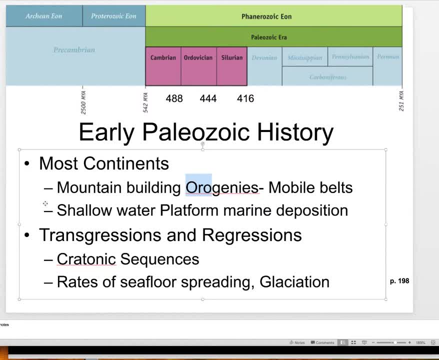 We also find that in the early Cambrian we see a lot of shallow water deposition. Remember the platform are going to be the younger sediments, mostly the Phanerozoic sediments, those that go into this Phanerozoic Eon. 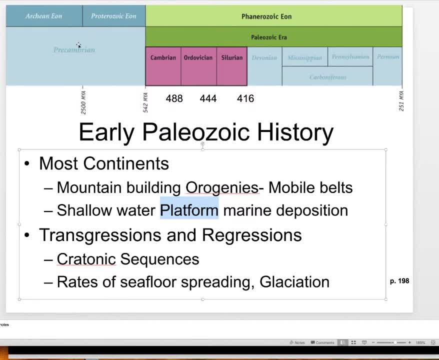 that overlie the Craton sediments, which are the pre-Cambrian rocks over here, And so we'll see mainly marine deposition even on the continent, which means we're going to have these, these shallow continental seas, which we call epicontinental seas, or your book here calls them. 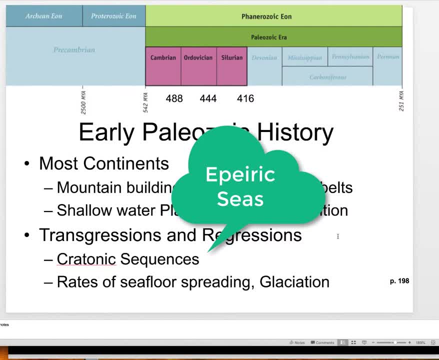 Epiric seas, So we'll get to those in a moment And really, because we have this shallow continent with few mountain ranges, to begin with in the Cambrian, we're going to see sea level fluctuations, transgressions, where sea level rises. 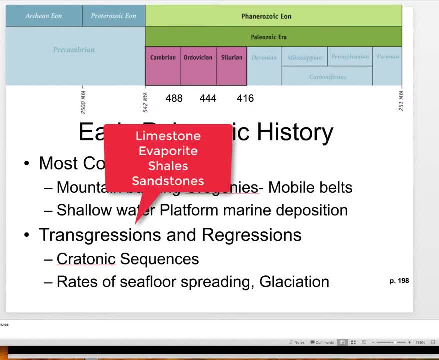 And when we see a transgression, we see a deposition of rock units, sandstones, limestones, evaporites, so we see the physical evidence. And then the regression is when sea level drops and it's usually that's marked by an unconformity, an erosion event, where we don't have the rock. 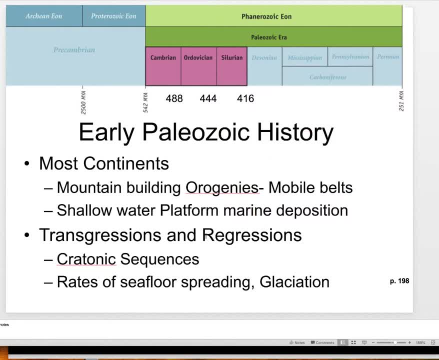 but we see that erosion event And so there's a time gap there, an unconformity. So, for the transgressions, we're going to break them out into these cratonic sequences, And there are four of these cratonic sequences in the Paleozoic that we'll talk about. 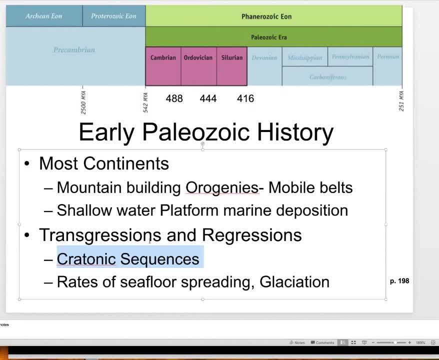 And then, what could be causing these changes in sea levels? Well, maybe we're seeing advances and retreats of glaciers. What we know is happening in the Paleozoic is Gondwana is forming in the Neoproterozoic to the Cretaceous. 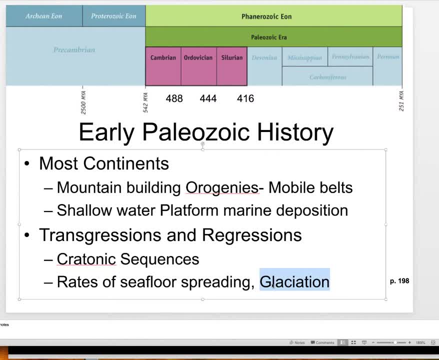 Early parts of the Paleozoic and it's moving over the South Pole. So glaciation is a key factor for sea level fluctuations, Also because we're rifting Rodinia and we're moving continental plates around by seafloor spreading. the faster the seafloor spreading, the higher the topography of the seafloor. 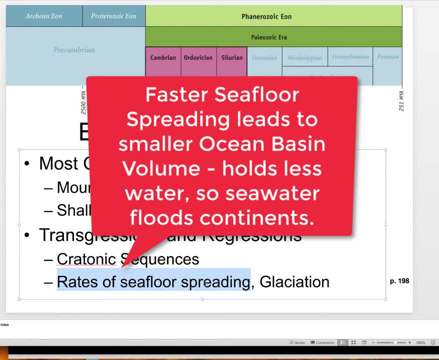 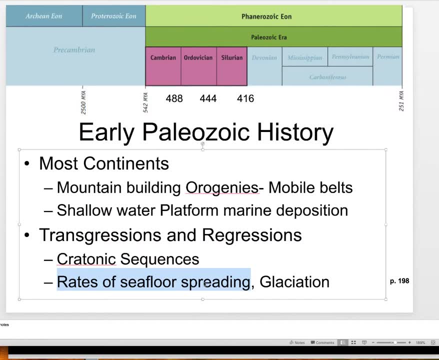 So if the seafloor topography is high, then it's going to push the seawater away onto the shores of continents, So it's going to increase sea levels. If the rate of seafloor spreading decreases, that means the seafloor will sink back down. 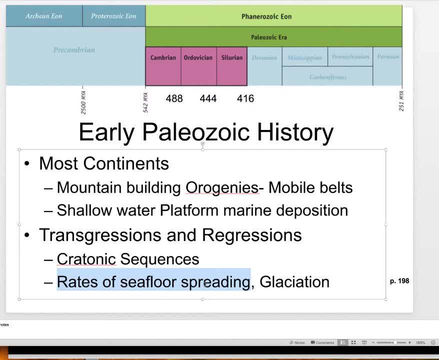 which makes the volume of the ocean basin larger. So the seas will retreat back into the ocean basin. So that's another way we can get these fluctuations in sea level. Let's look at the document camera here. So again, this Paleozoic Earth History, chapters 10 and 11.. 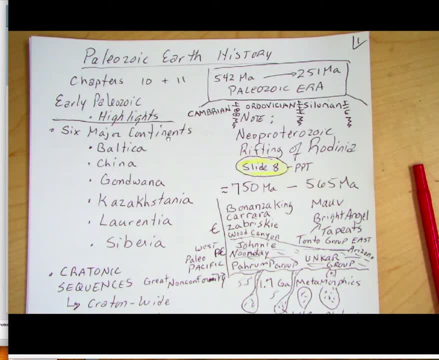 And some of the highlights. one thing that we will see in this chapter 10 is that the seafloor and the seafloor are very close to each other. So we can see that there are six major continents And really those continents developed because we had rifted Rodinia. 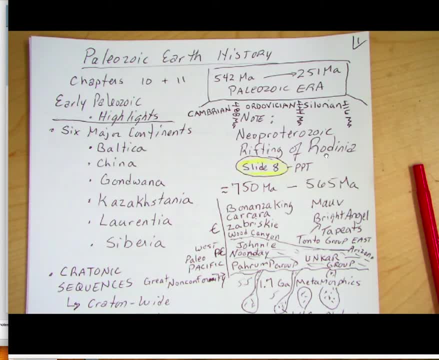 So in the Neoprotozoic time, between around 750 to about 565 million years ago, the supercontinent of Rodinia that formed during the Grenville Orogenes- remember, the Grenville Orogenes formed that supercontinent around a billion years ago. 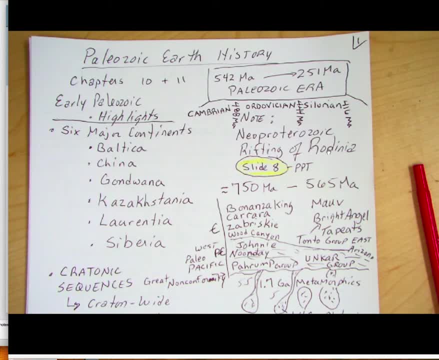 And then it rifted between 750 and 565 million years ago. So we have trailing continental margins on most continents right. And so the six major continents that were rifted out of Rodinia include Baltica, which is primarily Europe, and Russia west of the Ural Mountains, China, Gondwana, which is 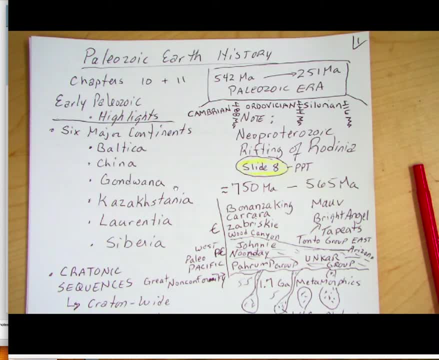 mostly the southern hemisphere continents- Remember Gondwana- is forming during this time, between around 750, 650 to about 500 million years ago, those Pan-African Orogenes that we talked about, And then a little microcontinent of Kazakhstan. 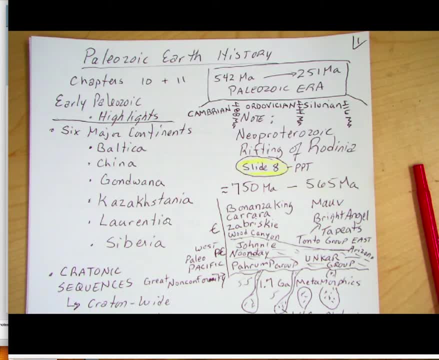 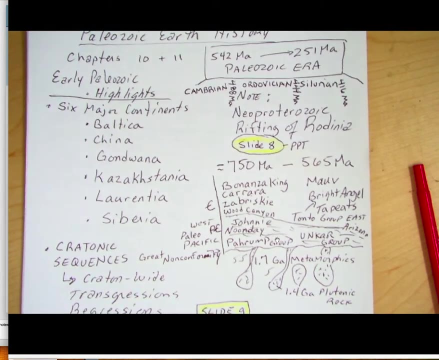 Cossackstania, Laurentia- important because Laurentia is North America, Greenland, parts of Scotland and Scandinavia, And Siberia is another continent that was around those times, Going back to this rifting of Rodinia. So during this time, remember, we're seeing this percambrian basement, which is about 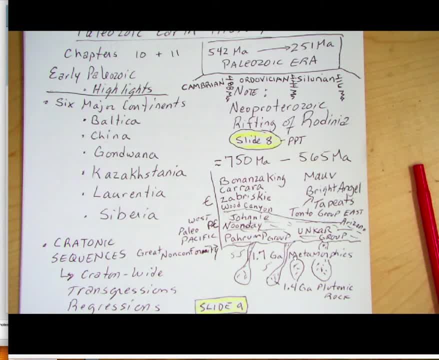 1.7 billion years old. We have those metamorphic rocks. If you think about the Grand Canyon. we have that Vishnu Schist Over in Death Valley. we see the Badwater, Nices And the metamorphic core complexes. 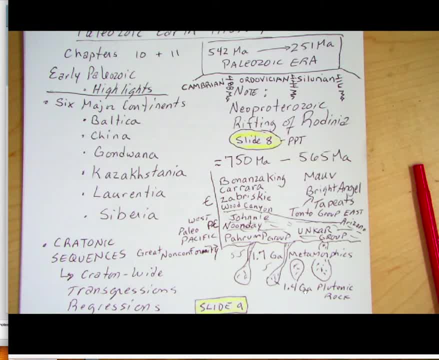 And they're all intruded by these 1.4 to 1.2 billion-year-old plutonic rocks. Remember, in the Grand Canyon it's the Zoroaster Granite, And we have some intrusive in the Death Valley regions that also date between 1.2 and 1.4. 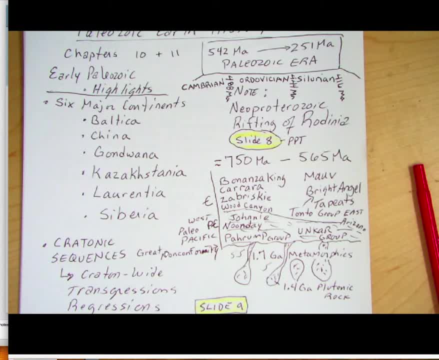 billion years. And then we have this kind of Creighton-wide unconformity, In fact we call it the Great Nonconformity. And in the Grand Canyon, remember, we have that Unkar Group which documents the first sediments on this great. 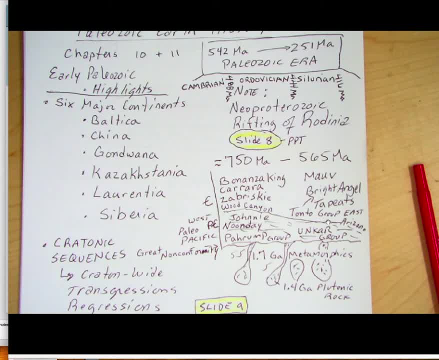 Unconformity here in Arizona. And then above that we start seeing the Cambrian. So this symbol here, a C with a line through it, means Cambrian. So for the Cambrian we start seeing that Tonto Group which includes the Taupits, the 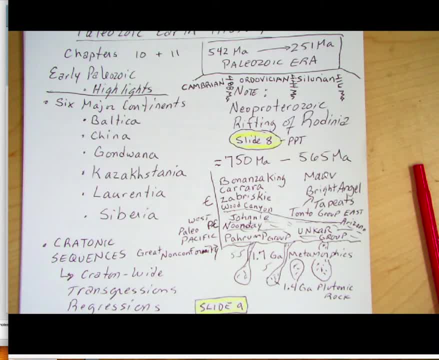 Taupit Sandstone, the Brighton Little Shale, the Mauve, Limestone- So we talked a little bit about these already. But while these are forming in the Grand Canyon of Arizona, over here in Death Valley we're seeing Cambrian rocks. 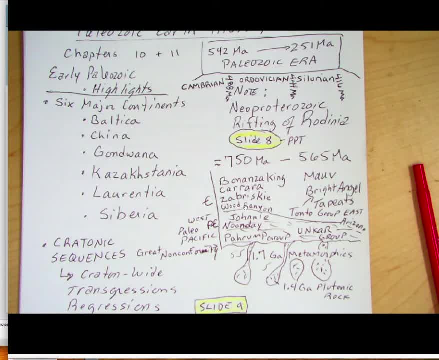 In fact, this Wood Canyon Formation is a limestone that really spans it, The pre-Cambrian Cambrian boundary here right. Then we see the Zabriskie Quartzsite, the Carrara Formation, which are a series of limestones. 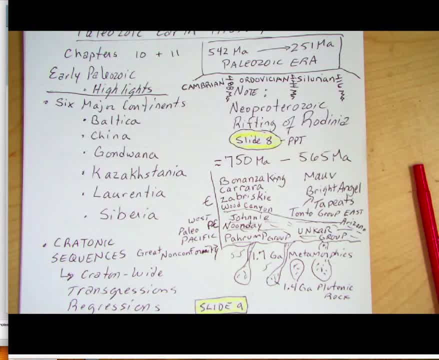 and some fine sands, And then the Bonanza King Formation, which is another series of limestones. So mostly we're seeing limestones- minor silicic, classic rocks- over here in the West, over in the Death Valley region, But at the same time we're seeing sandstones a shallow shoreline over in Arizona. 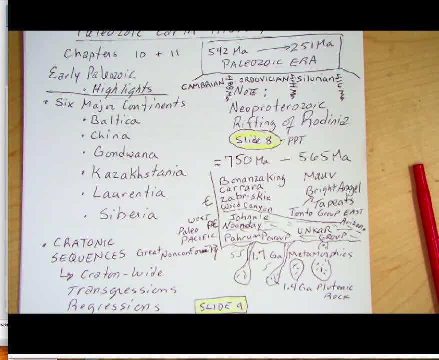 And then it gets deeper because we start seeing the Brighton Little Shale right, So top pieces of sand shale and then we get deeper with the Jamoff. So that's recording one of these transgression events right Sea levels getting deeper. 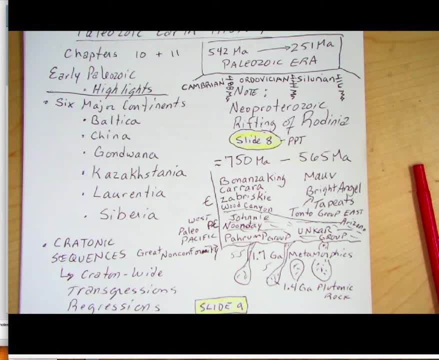 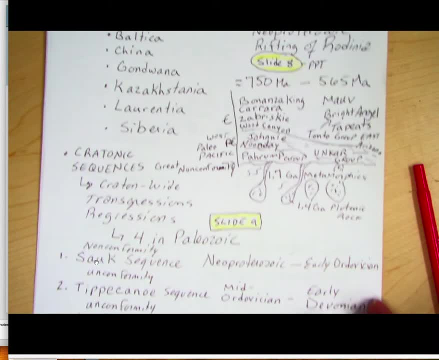 And you'll see, that's one of these first Creighton-wide sequences, or cretonic sequences, And that first one's going to be called the Sauk Sequence, as you'll see in a moment. Another highlight of this early Paleozoic time, or really throughout the Paleozoic 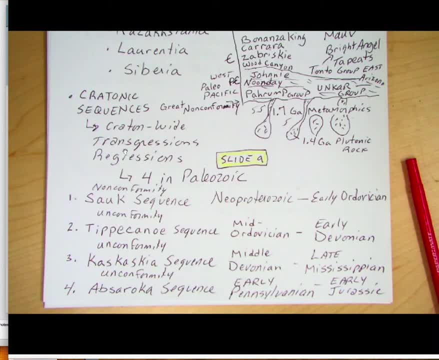 is. we do see these Creighton-wide sequences where we see sea level transgress over the continent, Which means we're going to start seeing deposition of sandstone, Then on top of that shale, Then on top of that limestone, Which is telling us that the sea level is getting deeper at that particular location. 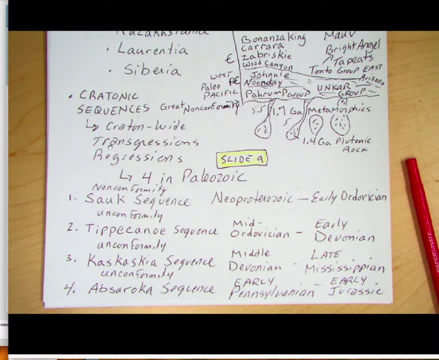 which means sea levels are advancing across continents And that's where we're getting these shallow epicontinental or epiric seas. And then there's going to be a regression where that sea level drops right. Maybe a glaciation event initiates or sea level or seafloor. 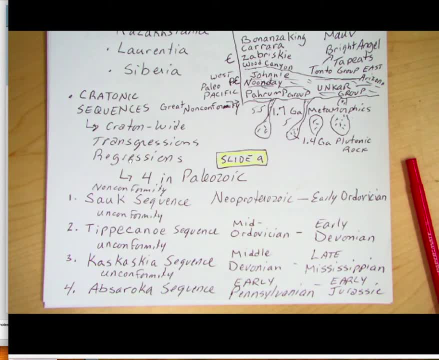 spreading rates decrease, But anyways, sea level drops and we'll see an erosion event that marks a regression. And in this Paleozoic time we're going to see four of these cretonic sequences. The first one, which is over that first, nonconformity, which includes the Tapeats. 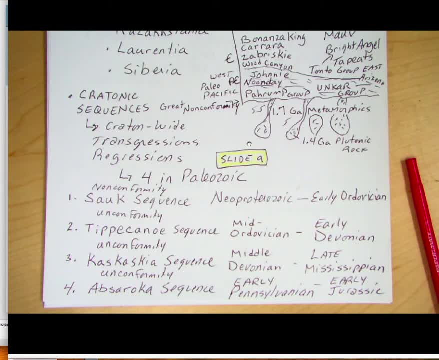 Bright Angel Moab or these formations here in the Grand Canyon region. Well, that's called the Sauk Sequence And that Sauk Sequence is neoperozoic from around maybe 600 million years early. Ordovician right. 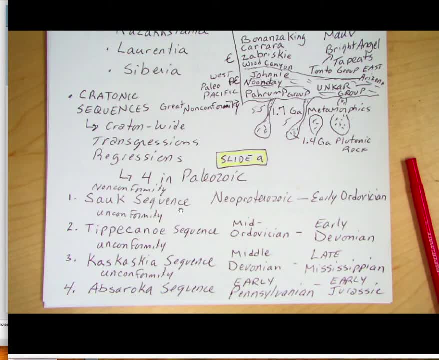 So neoperozoic to early Ordovician, and then there's an unconformity because there's a regression, And then the next sequence is another advance of sea level called the Tippecanoe Sequence, which is mid-Ordovician to early Devonian. 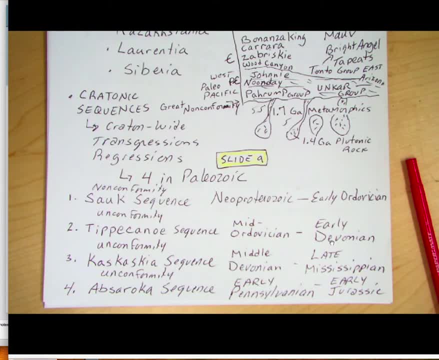 And so we there. we see a different type of sedimentary rocks being deposited, And then the sea level regresses and we see another erosion, unconformity event And the sea level advances again in the Kaskaskian time or the Kaskaskian Sea. 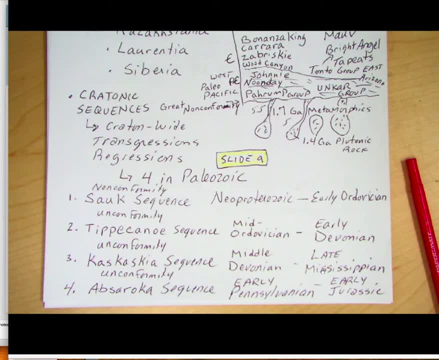 and that's going to be middle Devonian to� late Mississippian. but then there's another retreat of sea level and another erosion or conformity event here and then finally, the last Paleozoic advance of sea level is the Absarica Sea or the Absarica Sequence, and that one is early Pennsylvania and it actually 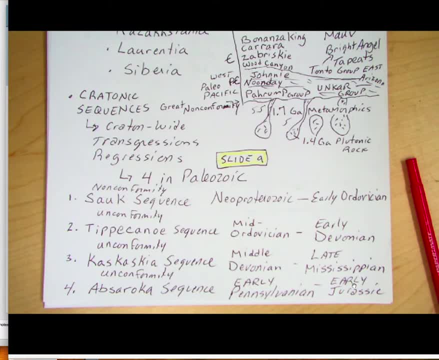 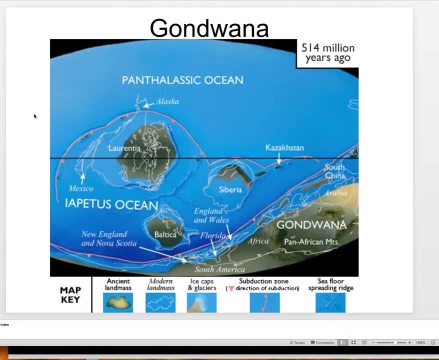 goes into the early Jurassic, which is part of the Mesozoic period. So let's go over here and look at slide nine, and this kind of will relate a little bit to what we're seeing here with this Sauk Sequence. So, looking here at this slide eight on the PowerPoint, I want you to know here this: 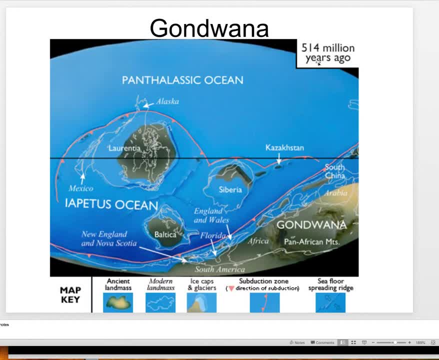 is Laurentia and during this time, around 514 million years ago, which is Cambrian time, we have North America, Laurentia, which is east-west, and note that the equator is pretty much going through the Great Lakes, Texas. over here, Death Valley region is pretty much. 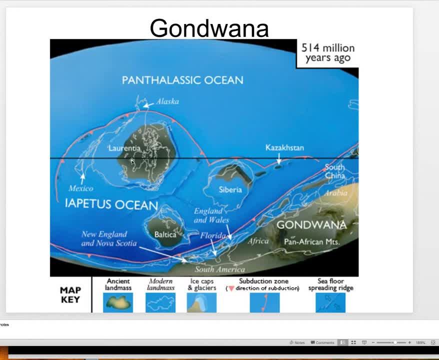 at the equator. the east coast of the US is pretty much south of the equator during this time, And then you'll see that over or during the Paleozoic period or eon, you'll see that Laurentia is going to do a counterclockwise rotation, so that it's going to be north-south. 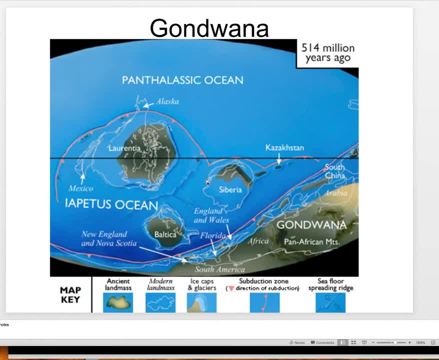 the way it is today. Highlights to note here is that when we rifted Rodinia, you know, Baltica spread away, Siberia spread away, Antarctica spread away. we opened up an ocean between Laurentia, Siberia and Baltica. 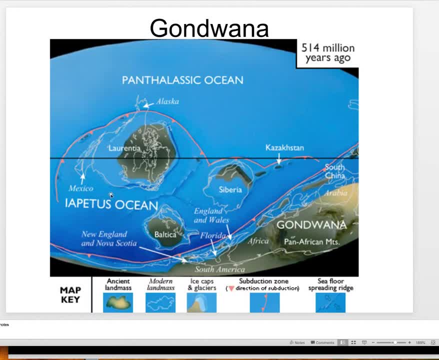 Remember, Baltica is going to be Europe primarily And that ocean that opened up here is called the Iapetus Ocean. So this is like the Paleo-Atlantic Ocean, This Iapetus Ocean, because eventually we're going to close this ocean and then reopen. 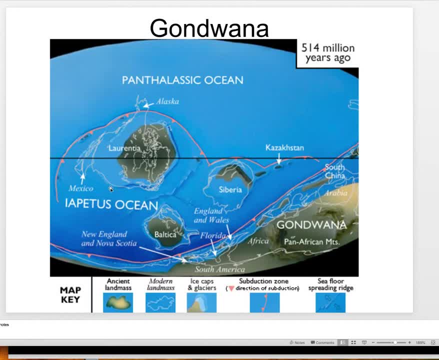 it to form the Atlantic. So, anyways, we have this stable platform and in this region we're going to form that Sock Sequence. This sea will advance across the continent, this shallow epi-continental sea, depositing those units that are characteristic of the Sock Sequence. 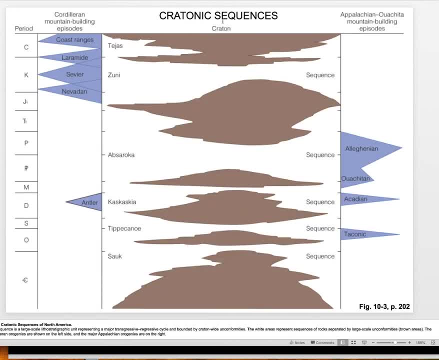 Now, when we look at these cratonic sequences, note that we want to look at what's going on here. So this symbol again means Cambrian, Ordovician, Silurian, Devonian, And so that Sock Sequence again is going to be from the Neo-Protozoic to about the Mid-Ordovician. 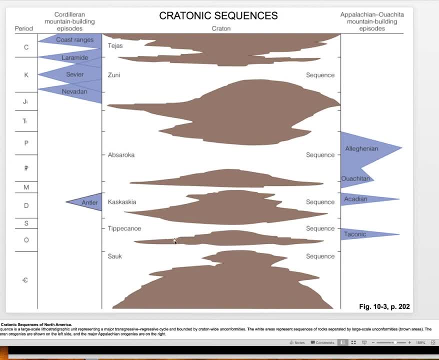 And then there's going to be this Creighton-wide unconformity or erosion event, which is a regression, And that's our Tippecanoe Sequence. we'll come after that, And then there's another regression here, and then, well, that's the advance of Kaskaskia. 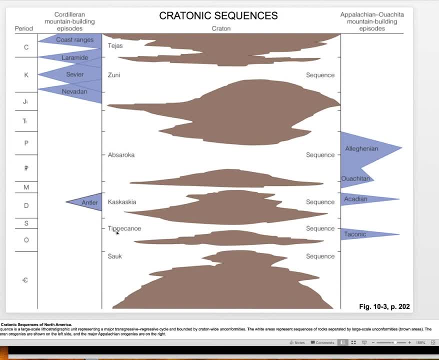 Sea. So, anyways, this kind of documents, those at least the four that we see in the Paleozoic, And then there's another regression here, and then, well, that's the advance of Kaskaskia Sea. So, anyways, this kind of documents, those at least the four that we see in the Paleozoic, And then there's another regression here, and then, well, that's the advance of Kaskaskia Sea. And then there's another regression here, and then, well, that's the advance of Kaskaskia Sea. And then there's another regression here, and then, well, that's the advance of Kaskaskia Sea.